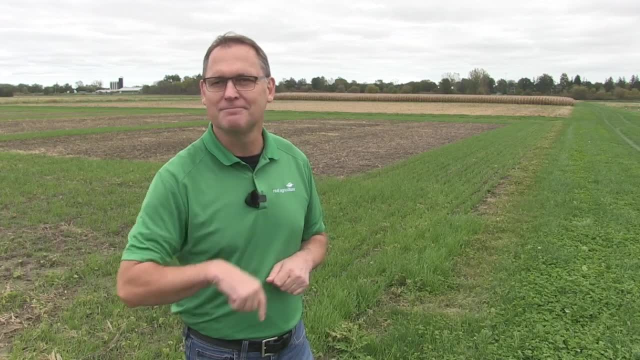 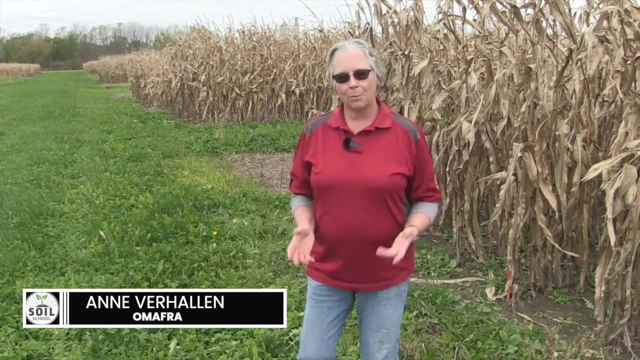 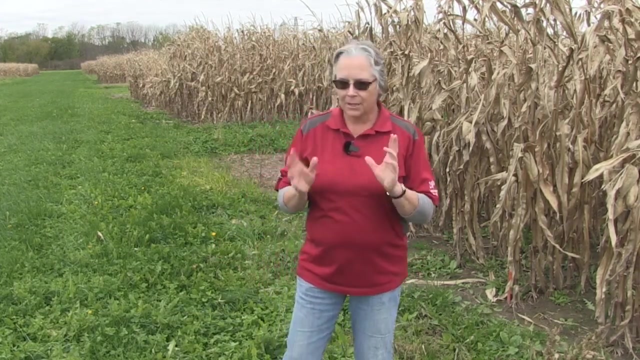 with how you manage that soil. Here's Anne Verhallen. So what makes a healthy soil? That is the eternal question, right, And it's a tough one because it really depends. It depends on how you define soil health and depends on the soil type that you're dealing with. So let's take the soil health part and 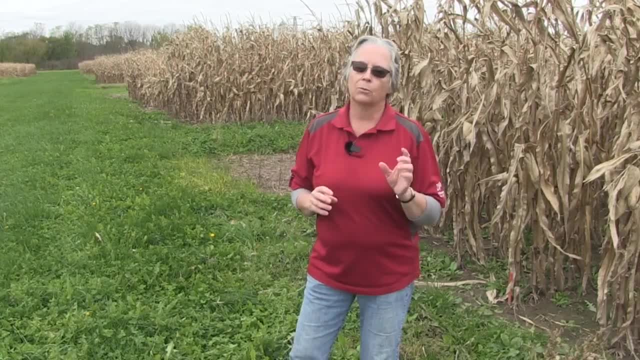 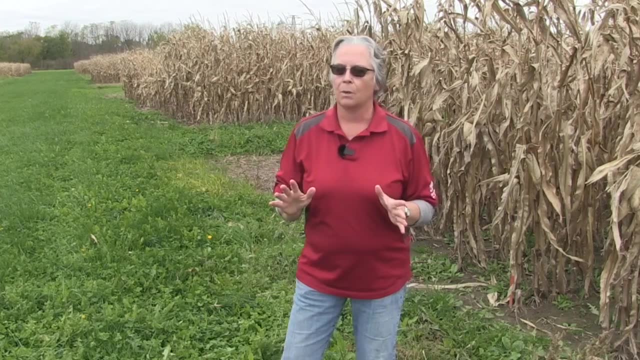 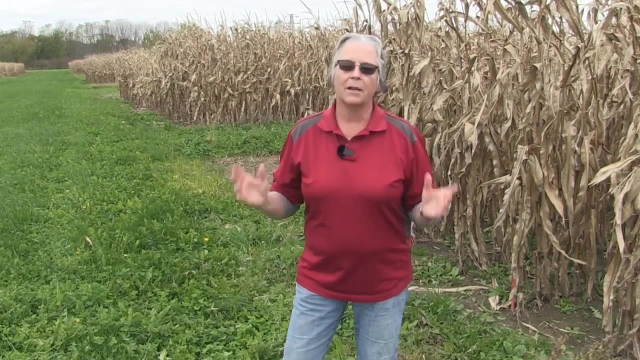 take it apart a little bit first. So we'll often hear the words soil health and soil quality used interchangeably, And in my mind they're not exactly the same. Soil health is. well, let's start with soil quality. Soil quality, to me, is the inherent properties of that soil. 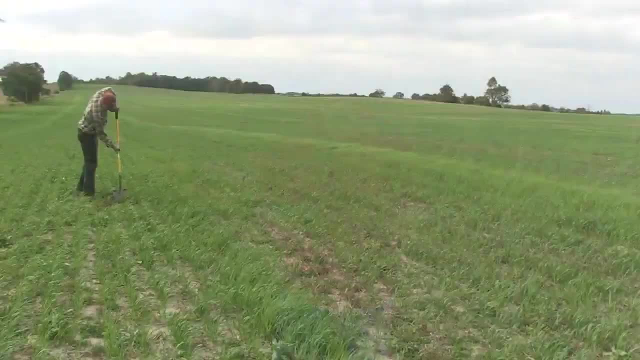 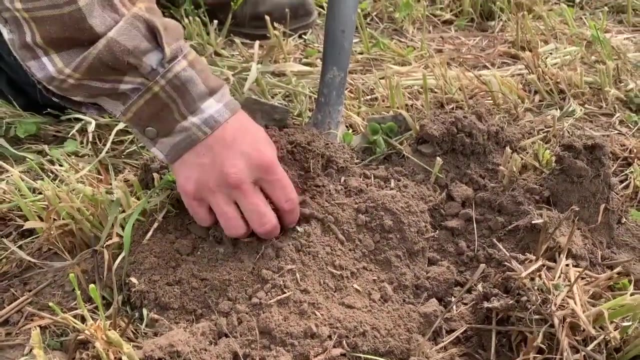 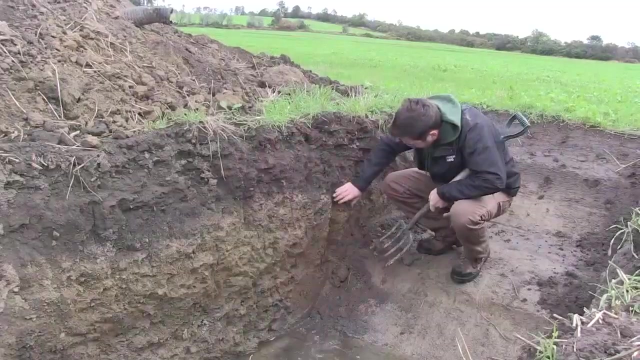 So is it a sand, Is it a silt, Is it a clay? Is it in southwestern Ontario Or is it in northern Ontario? So location matters, soil type matters, previous history and management matters, But a lot of the soil quality part really is the inherent quality. So it's: what's the soil profile like? 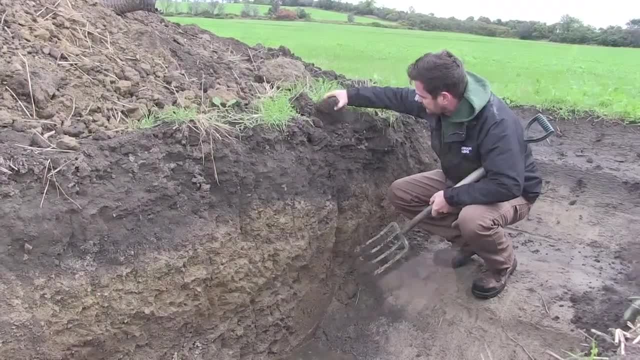 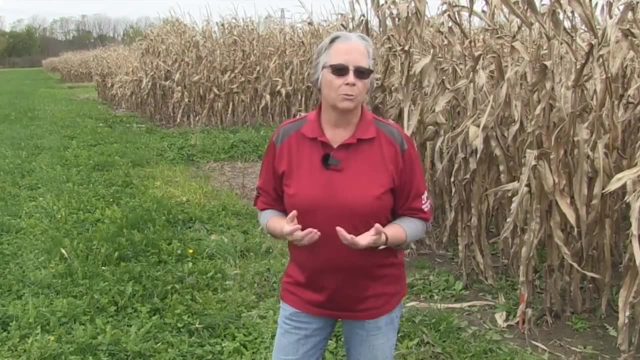 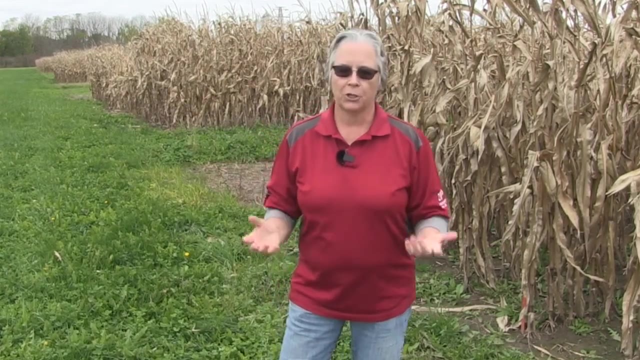 What's the internal drainage, Whereas soil health is. how is it managed And is it reaching its full potential? An example I often use is: if you think in terms of human health, you're talking about a human health. So, using me as an example, my quality would be my genetic component. the fact 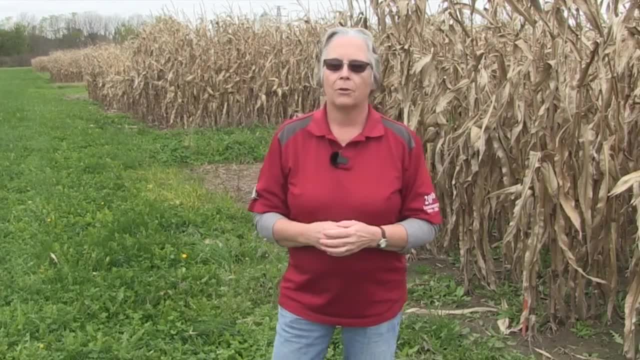 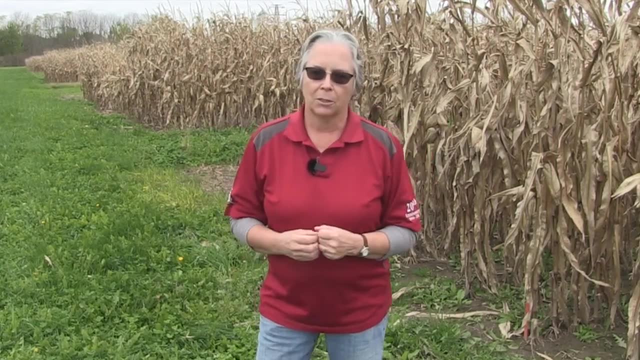 that I have a father who had a heart attack at age 50. There's cancer in my family. all those great, wonderful things to look forward to, And the fact that I'm living in southwestern Ontario with some of the poorest air quality in the country. So that's my quality. My health is how well I manage. 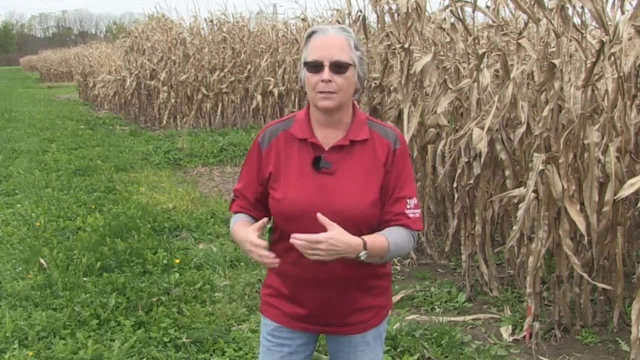 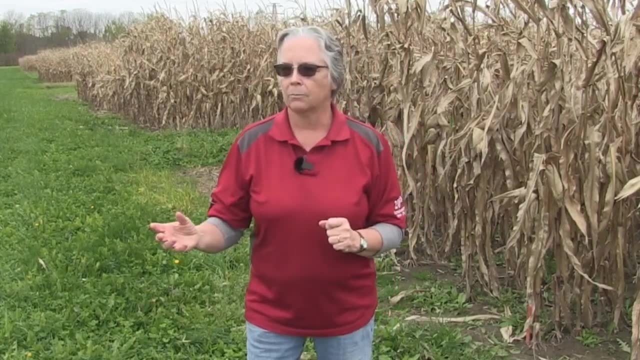 that And how healthy I am because of that. So my exercise, my diet, how I manage my life, So it's the same kind of thing when we talk about soil health versus soil quality. So the next part: if we're thinking about soil health, we usually talk about it in 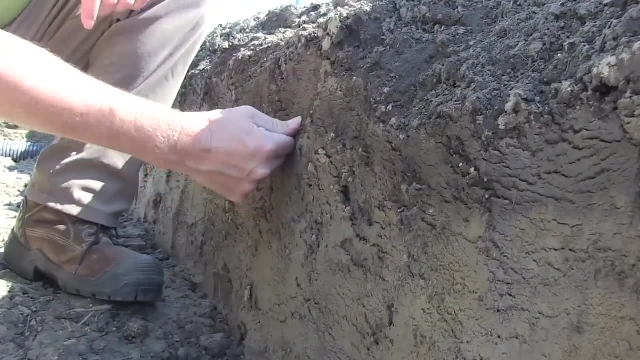 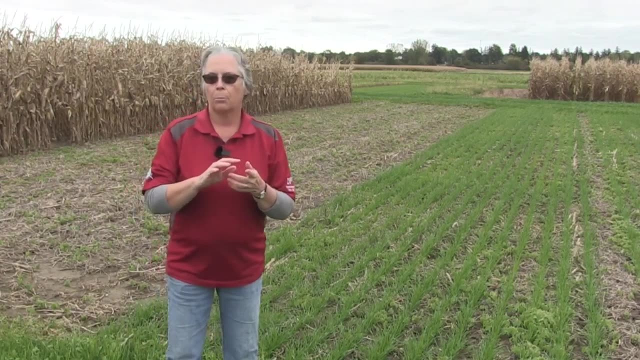 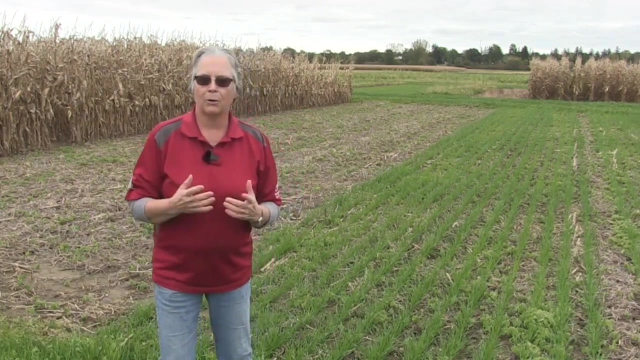 kind of three pillars or three groupings, One being chemical, So that's our fertility and pH. I think we've got a pretty good handle on that. Then there's biological. That remains a bit of a black hole. There's lots of study being done, But it's micro, it's. 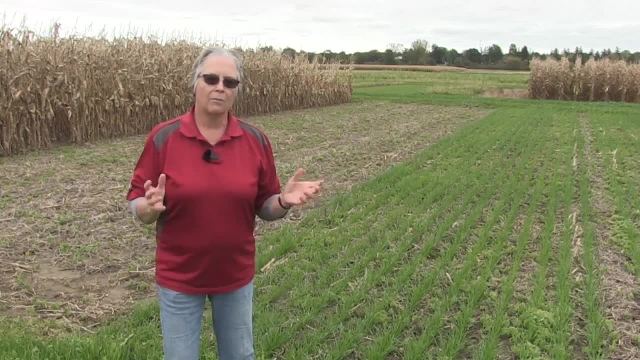 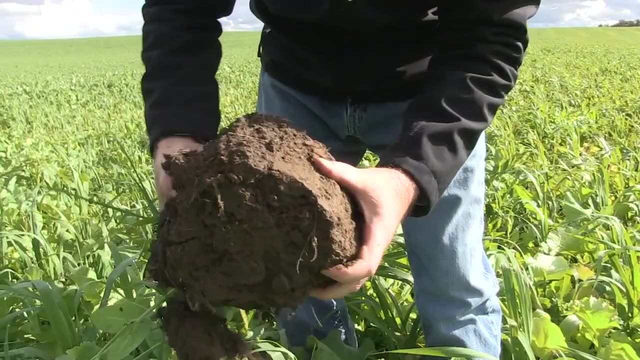 from microbes to earthworms and ground beetles. So there's a lot of unknowns there. And then the third part is the physical. So this is the structure of the soil, How those aggregates, how those soil particles are held together in aggregates and how those 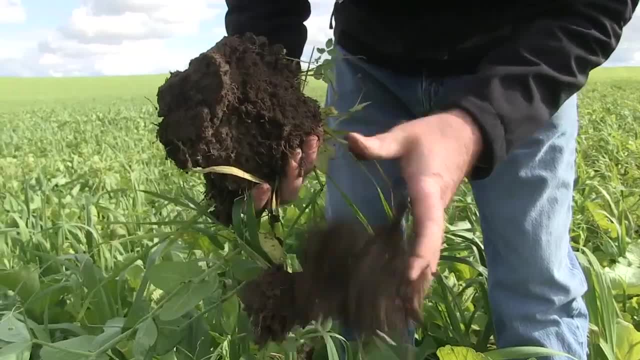 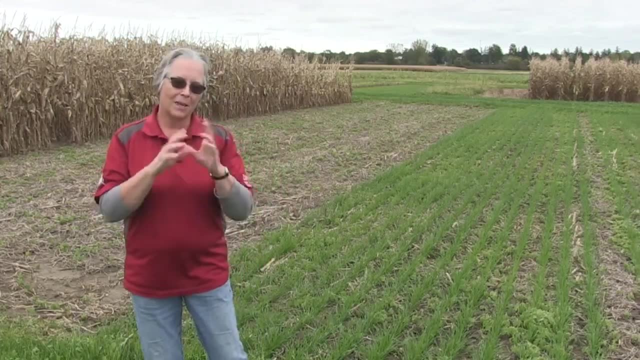 aggregates are held together in terms of making good tilth and a good soil structure to grow crops in. So the thing that binds all this together, though, the thing that is shared by all three of those pillars, is organic matter, or carbon, depending on which way you want to put it. 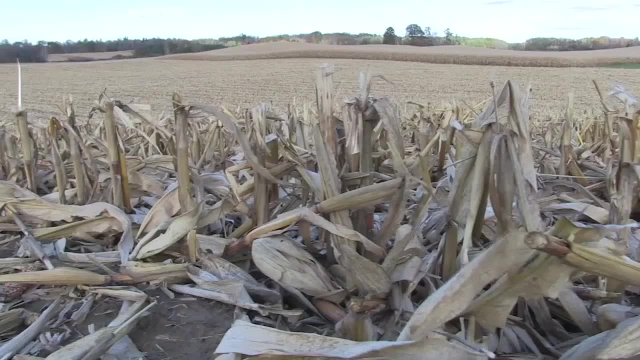 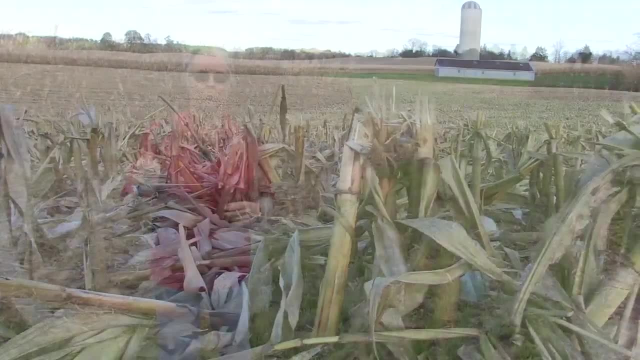 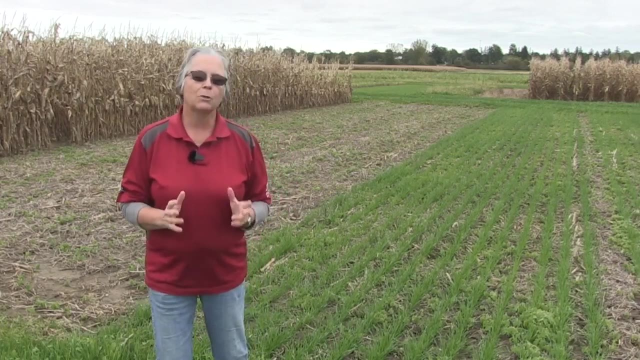 I'm going to talk about it. And organic matter is the binder, It's the piece that helps to hold fertility, It's the piece that is part of the biology and also drives biology. And then, with the structure, organic matter, organic carbon, plays a huge role in building a stable structure. 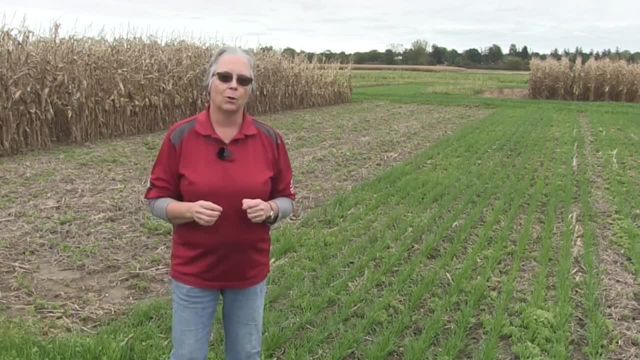 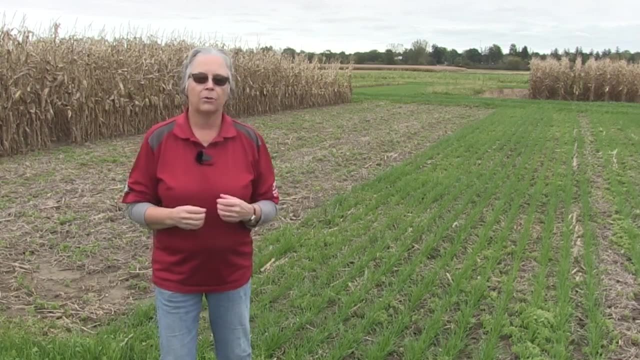 And a stable structure is really what we're looking for in a healthy soil. We're looking for a porous, open soil that allows plant roots to thrive, for the seed to adjust- And that's what germinate establish- and then those roots to be able to scavenge through the whole soil profile. 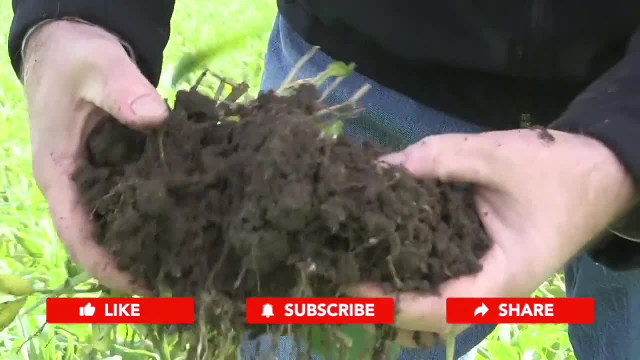 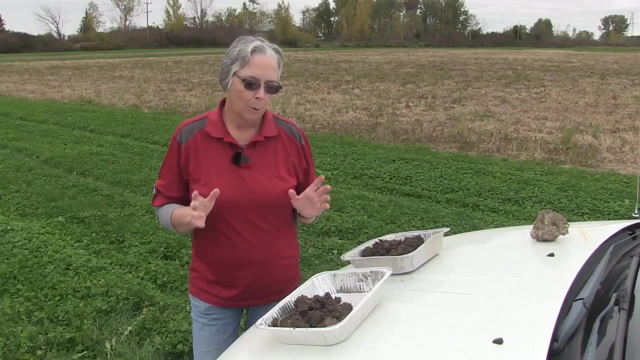 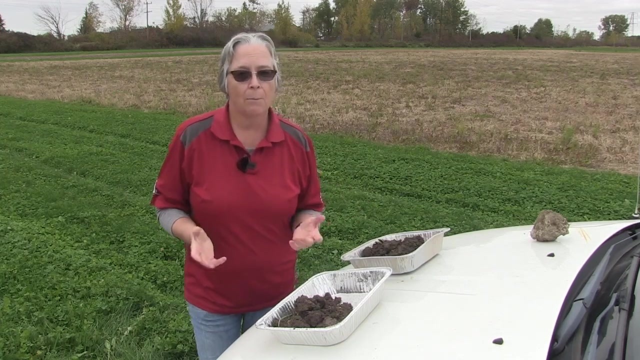 that's what we're looking for in a well-structured, healthy soil. so 2021. it's been a terrible wet year, but different soils have taken it differently and a lot of that comes back to, of course, soil type and and drainage, but a lot of it does come back to 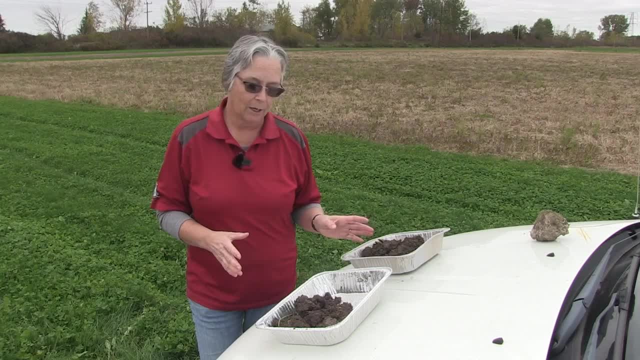 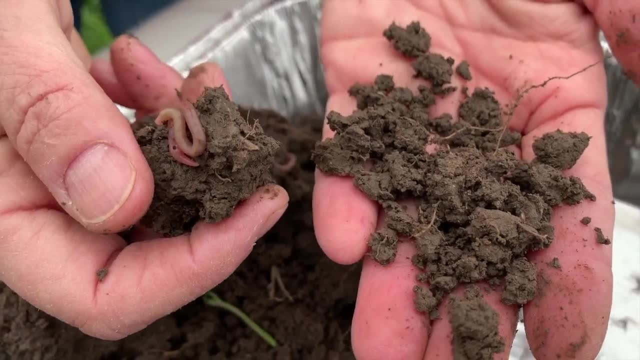 soil health. so let's take a look at these two samples i've got here. this first one here is a field that's got a diverse rotation that also includes perennial forages, and i can already hear you guys saying i can't afford to grow forages. okay, fair enough, but i just want to. 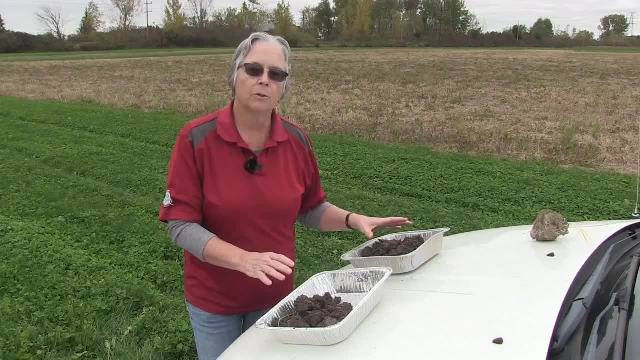 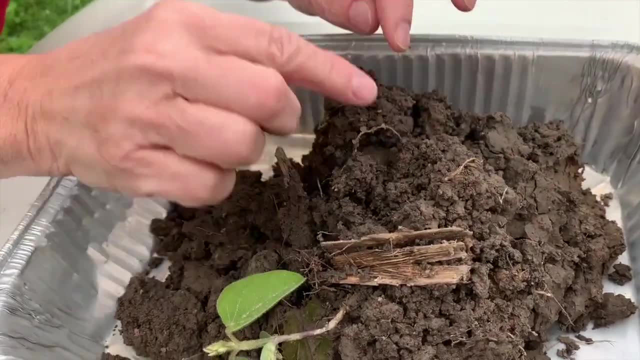 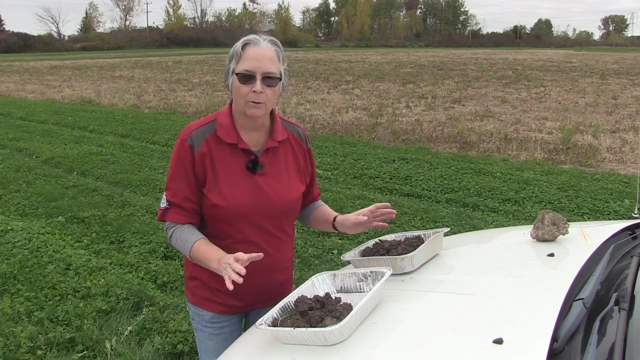 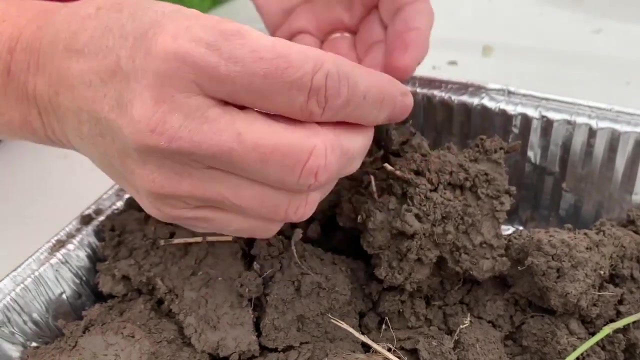 show you the difference. and this other field has a long-term rotation of corn, mostly corn, a little bit of beans and virtually no wheat. and what i see strongly structurally here- and admittedly they're both very wet samples because they've never dried out since july- what we see is tremendous structure. we've got these fine little aggregates with this. 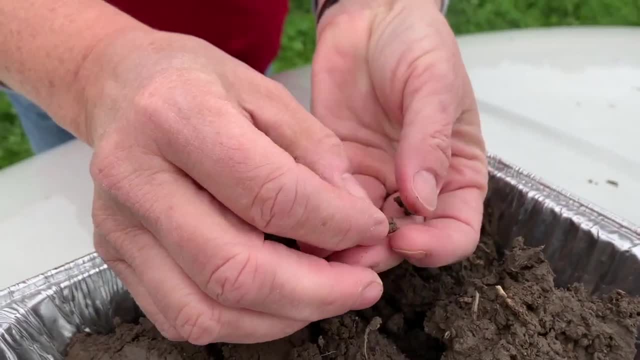 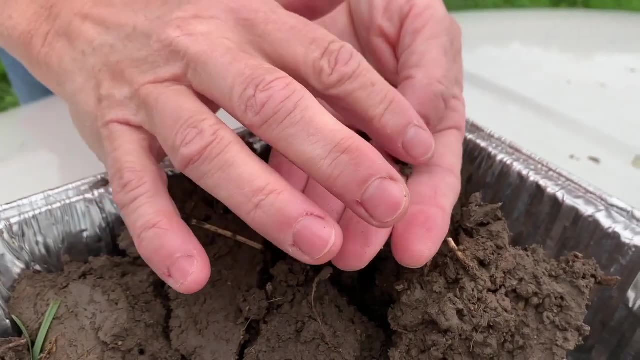 this field that's got the perennial forages in it, it's got a darker color. it actually has almost a point more organic matter. this is something around 4.3, whereas this other field and they are separated by less than 100 feet, so they are the same soil type. 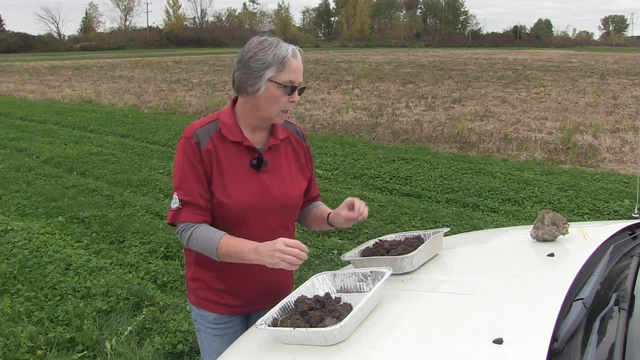 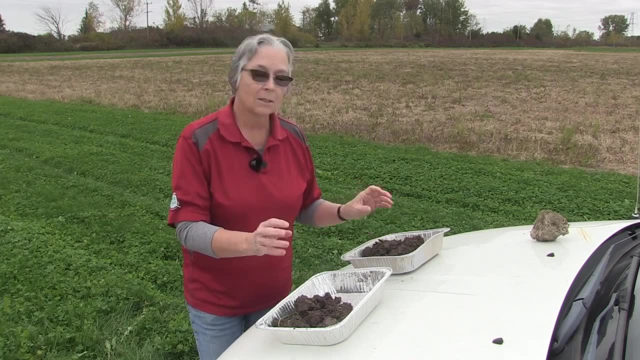 they are separated by less than 100 feet, so they are the same soil type. they are separated by less than 100 feet, so they are the same soil type. they've just been managed differently over the long term. this other field is somewhere in low three's. so about a point difference. in organic matter there's a slight color change even, but you 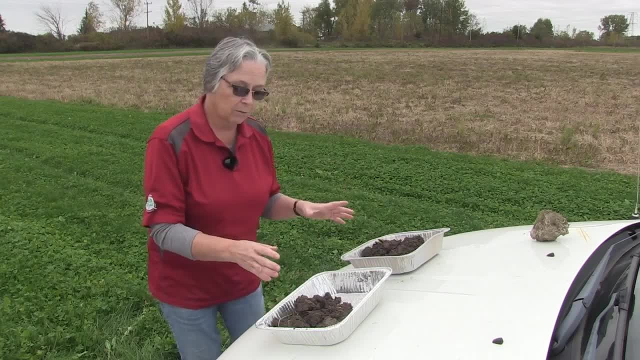 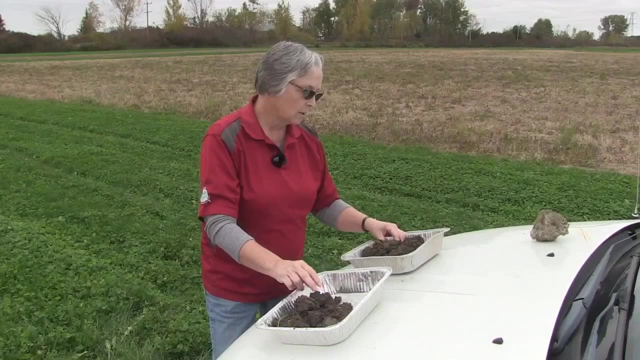 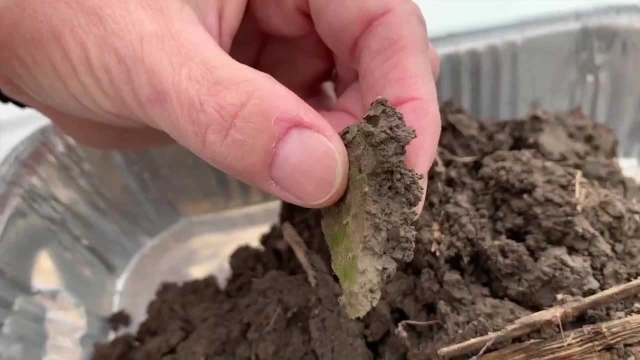 can see the difference in the surface of the soil. this surface is still quite open, it's. you can see the aggregation with it, whereas this field, the one that's been primarily corn, has been sealed and if it was a little bit drier you would see that in the soil. but once you gladiate this soil it actually 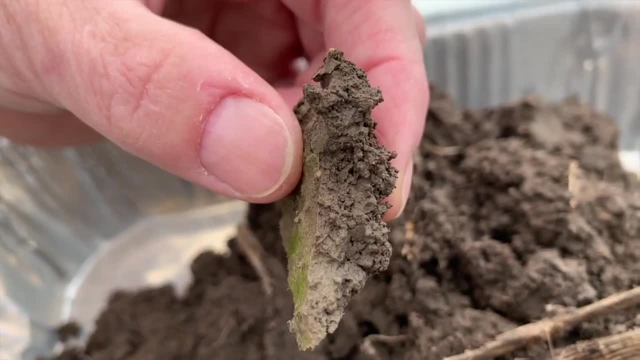 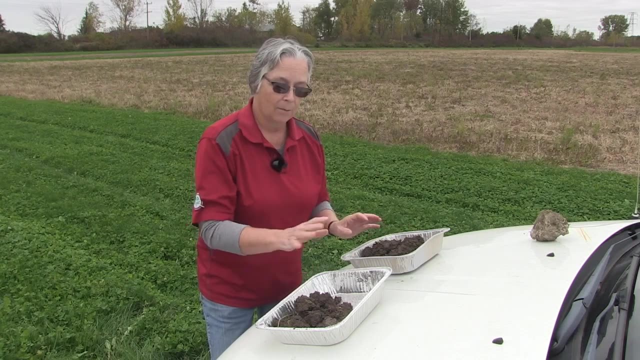 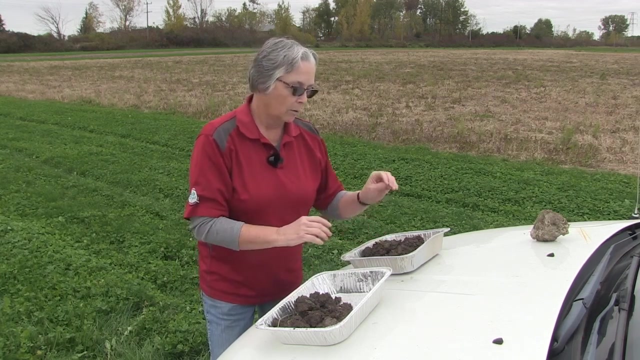 that we've got a very thick crust on it. they're both very productive soils, but one is more resilient than the other. this one with the higher organic matter, the better soil structure, is going to be more resilient year in, year out. this field, yeah, it is very productive. but take a look at a 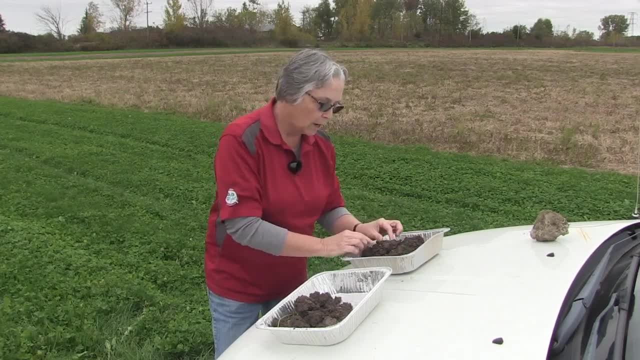 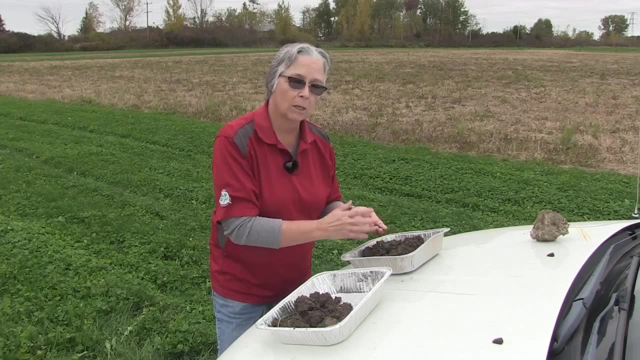 couple of things. one, we've got the ceiling at the surface. we do have these fine aggregates which if i threw into water, you're going to find that they're not water stable, so they're going to blow apart. that's part of the reason we're getting the ceiling at the surface. and then when we look, 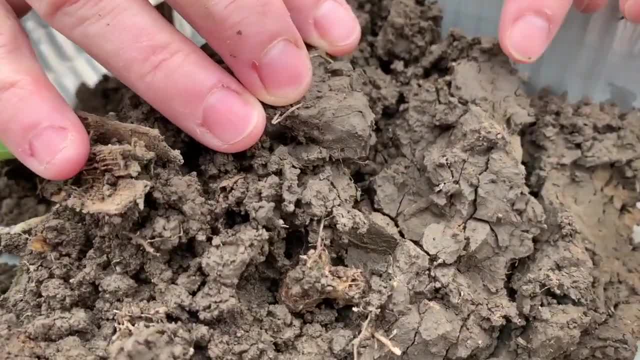 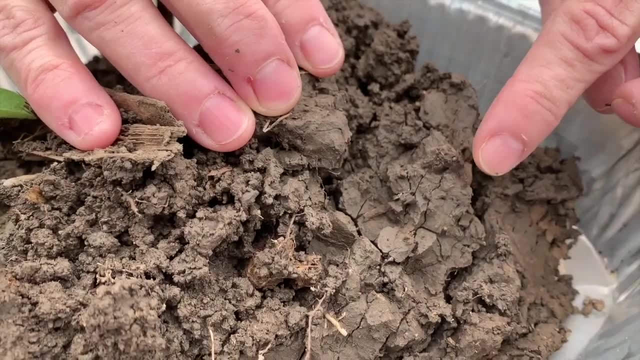 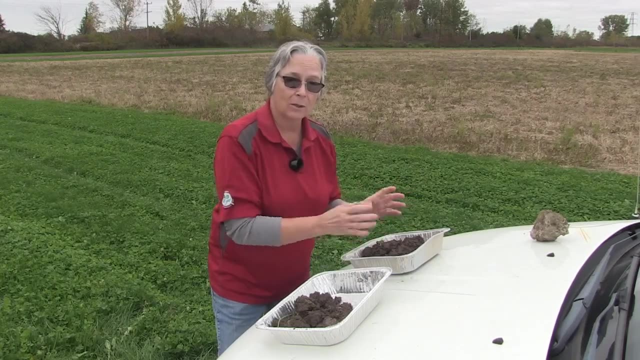 further down into the, the just below the tillage pan, you can see that we have a much more blocky type of structure with just very fine cracks. that's what we're depending on: getting the moisture, the excess moisture we've got right now from there down into the tile to deal with this. 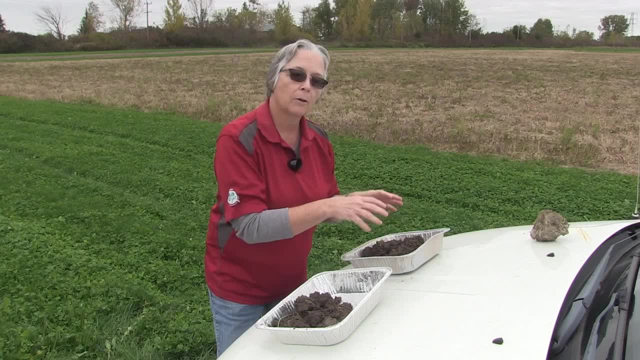 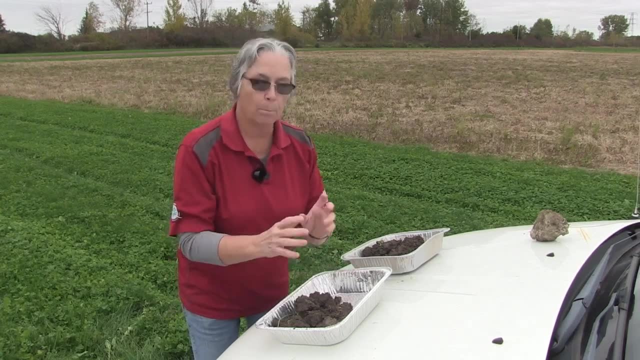 field. so we've got a problem in getting the ceiling at the surface. so we're going to have to make sure that we're getting water through this soil, whereas the wider rotation with the higher organic matter, the better structure. one is going to hold more water in years where we're dry and 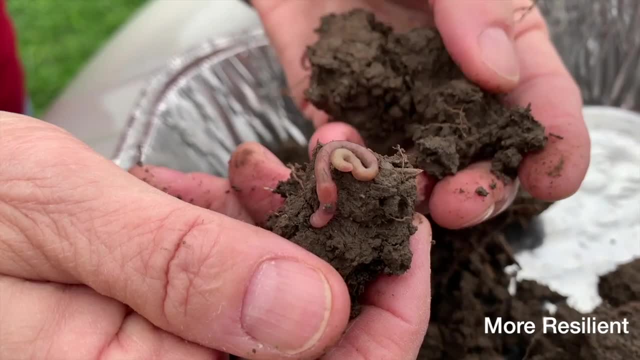 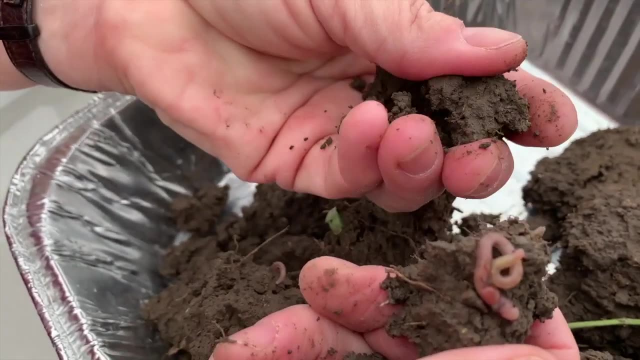 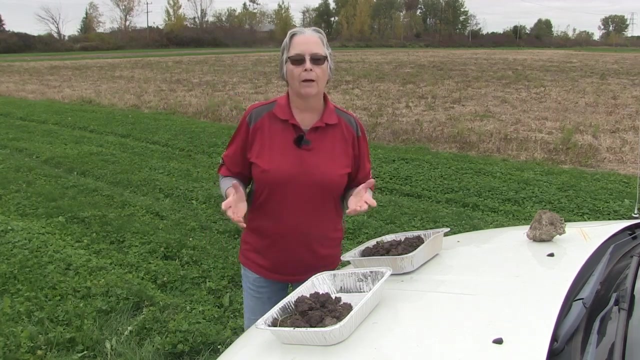 it's also going to let more water through. so more resilient, less resilient still, both very productive soils. these both can easily make over 200 bushel corn. so again, coming back to what makes a healthy soil, some of it is the background, it's the soil itself and what you're trying to do with it. but the other thing